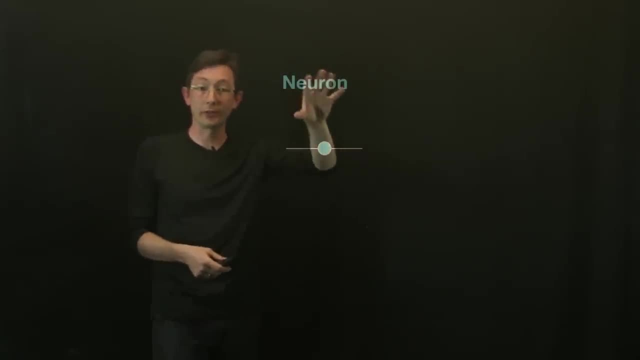 So the basic building block of a neural network is a neuron, which is this little functional unit, kind of an input-output node or neuron, And, to be mathematically precise, you have kind of an input signal u that goes into this node and it does some mathematical. 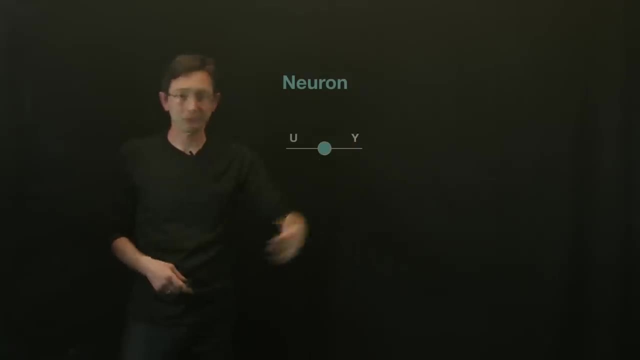 operation on u to give you some output y, And this could be something like just multiplying it by a constant or adding a constant, or it can be more sophisticated. So often people use sigmoidal functions. These are called activation functions, Where if u is small, the output is just zero, And if u is large, regardless of how large it is. 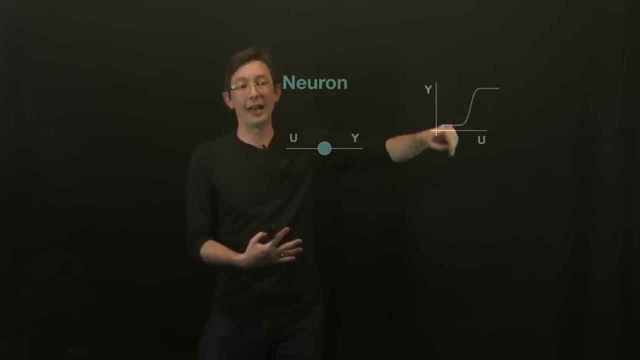 the output might be one. And then there's some smooth activation function from zero to one. This is a sigmoidal or a hyperbolic tangent activation function, Very, very common, Also neural-inspired, So a lot of the neurons in your brain kind of have these sigmoidal. 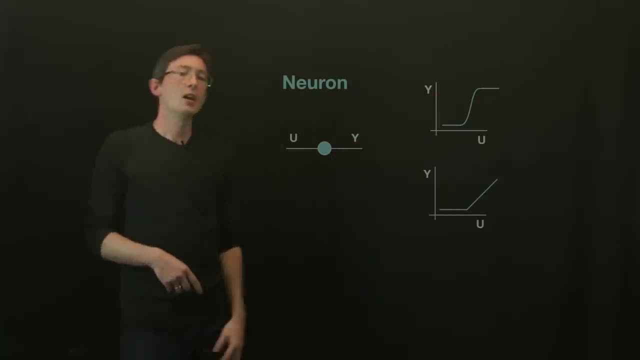 activation functions. So this is really really commonly used. Increasingly now people use this kind of this rel u linear kind of it's zero up until a point and then it grows linearly with u. This is a very useful building block that people are using in. 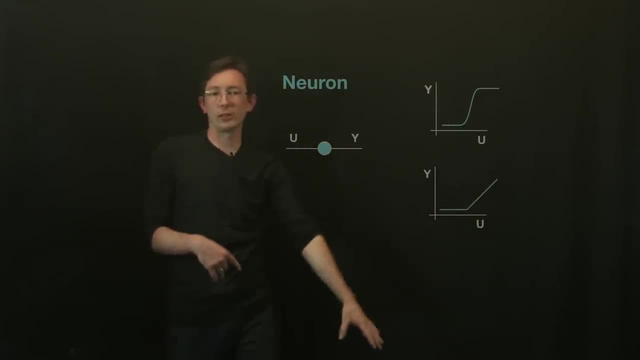 modern machine learning architecture, And I could give a whole lecture on all of these different activation functions. There's tons of them. Some are better for something, some are better for others. The rel? u is very common, so is the sigmoidal. 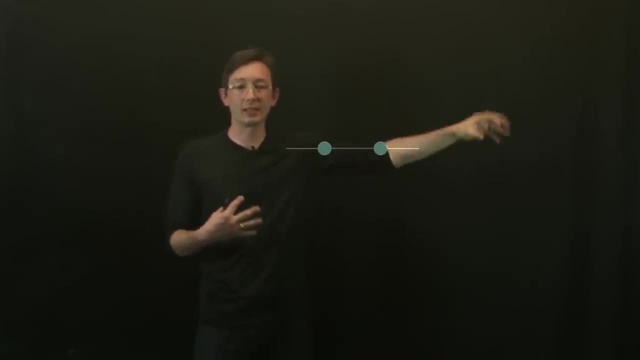 So you take that neuron, that unit, and you start to stack it, either in series or in parallel or both, So I can put two neurons next to each other and do a more complicated function, This function, followed by this function. I can have middle layers. I can, for example, do three different functions from this output. 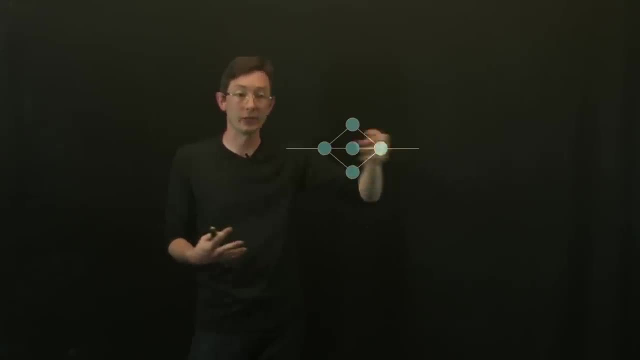 And then I can add all of those up or multiply them or do some other function downstream, And so I can build up this kind of complexity in what's known as an artificial neural network. So here I've built up this neural network. It's a network with nodes and edges describing the topology of how it's connected. 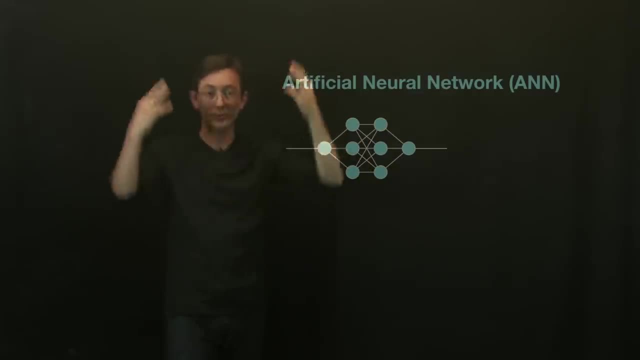 but it's artificial. So neural networks, you know you have neural networks in your head. This is an artificial one, built up out of these building blocks, And the different nodes can have different activation functions. They can add up linear combinations of the previous layer and things like that. 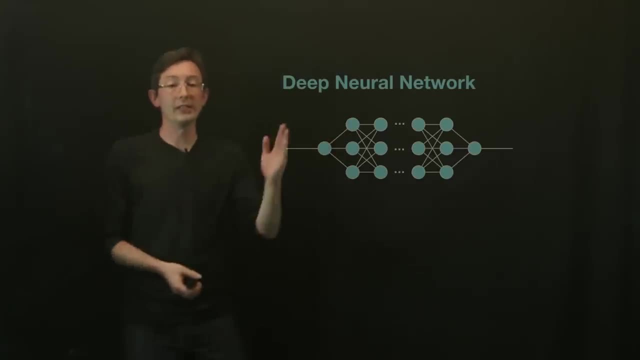 Okay. And then if you keep stacking more and more and more of these layers, so each layer is doing some kind of sequential processing, if you start to add a lot of these, then you have what's known as a deep neural network, And this is the basis of deep learning today. 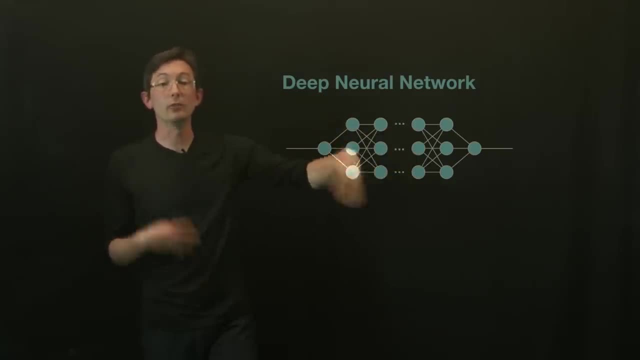 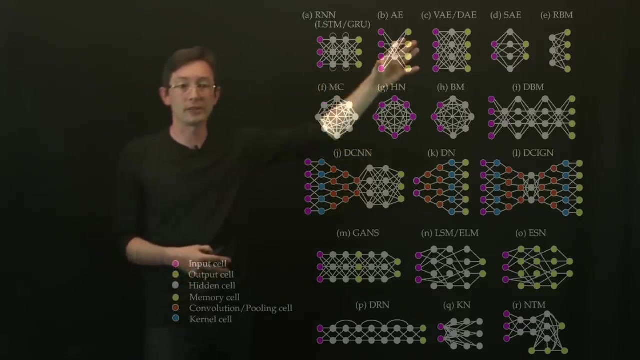 Okay, And so there are a ton of things you can do with these neural network architectures. I'm just going to show you a few here. So this is kind of the neural network zoo. My colleague, Nathan Kutz, made this image. It's inspired by the Asimov Institute's neural network zoo. 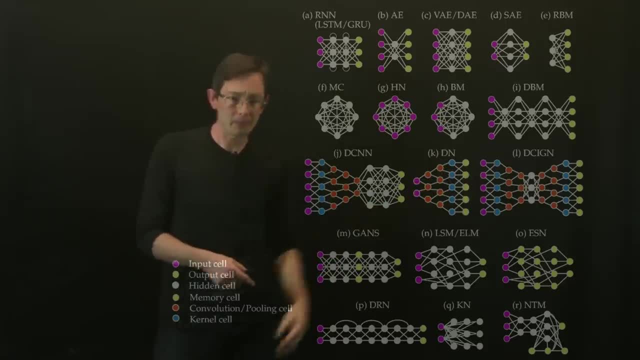 This is in our textbook Data-Driven Science and Engineering, And this just gives you an idea of some of the massive variety of neural network architectures that you can design, And so each color for the different nodes means different types of nodes, different types of computations that are happening. 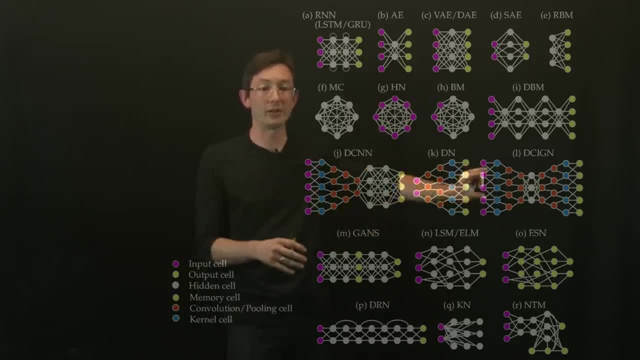 There's also the different topology of whether or not information is getting compressed in a bottleneck and expanded, or you know all of these different architectures- And this is only a few of kind of the architectures out there in neural networks. So really there are tons of different and every year there are dozens of new architectures being proposed to solve different problems. 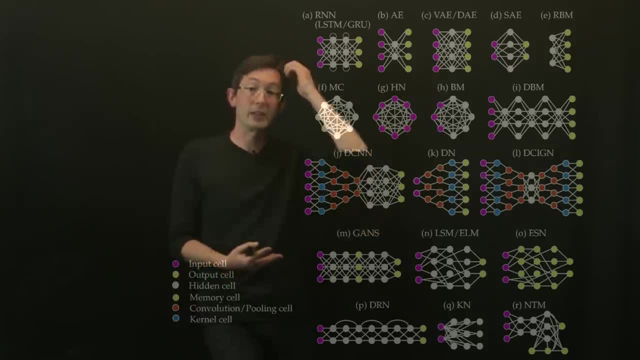 So it really is a zoo. There's a ton of different things you can do And we're increasingly learning, through trial and error and study and analysis and lots of hard work by many researchers, which architectures are good for which problems, And so, again, this is just a few of them. 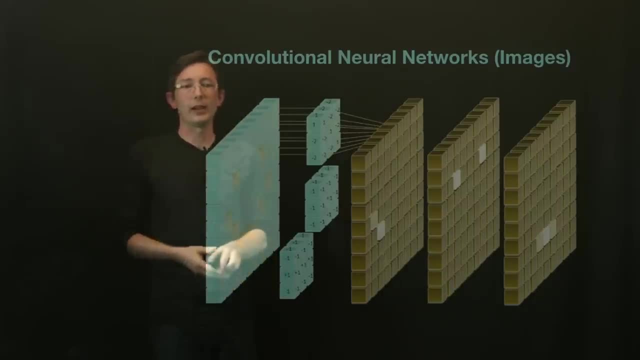 So a couple of key ones I want to point out. Convolutional neural networks, CNNs, are really, really important. These are used a lot in image recognition. The basic idea is, if I have a big image, this array here, I don't know if you can see, but there's a smiley face. 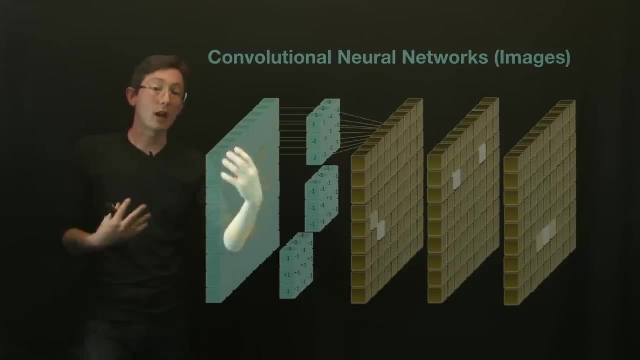 I took this from Wikipedia. What a convolutional neural network does is it has these convolutional layers that basically take a mask and slide it across the image, doing local computations in local patches, And so what you might be able to do is pull out edges or features. 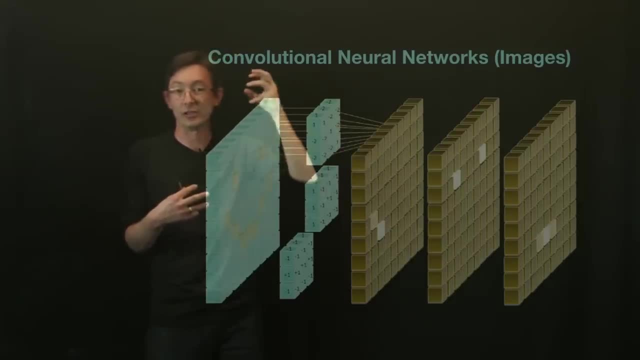 And you would run that through a convolutional layer and pull out these edges And then you might run those through another convolutional layer and another convolutional layer And you stack these convolutional layers and then you do some processing on them And so convolutional neural networks. CNNs are really important for image recognition. 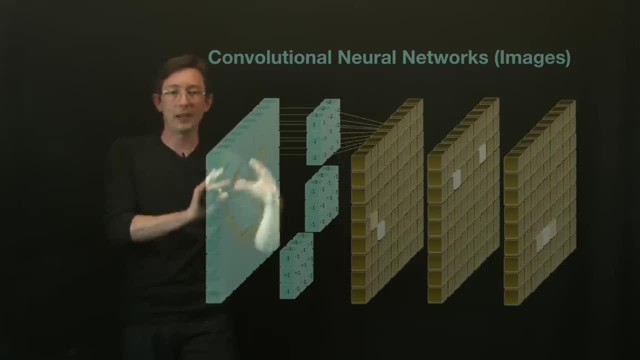 Anything where there is a translation invariant. So you know, if I have a picture, a picture of a cat, the cat could be over here, or it could be over here CNNs can start to pull out kind of this translational invariance that exists in images. 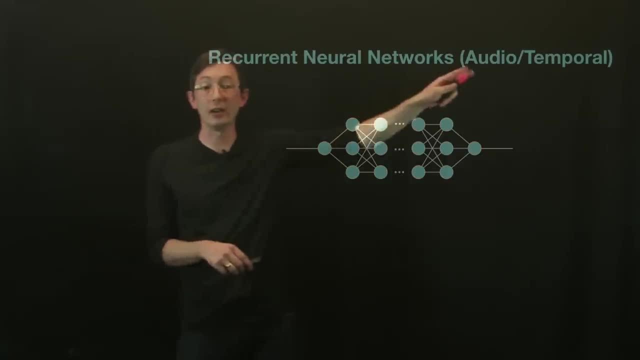 Recurrent neural networks are really useful for audio and temporal signals, signals that vary in time, like if you looked at the acoustic signature of speech in time And what these do. I didn't actually draw it, but what you can do is you can add these kind of feedback loops. 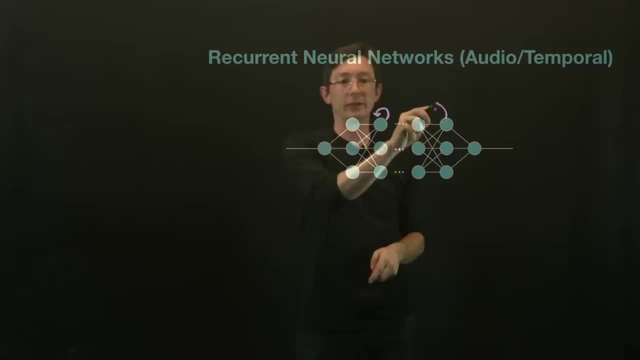 so you can have the neurons feeding back to themselves, Or I can have different layers kind of feeding back, And so this allows you to have this kind of temporal feedback where there's some memory in the system. It's not just a feed-forward network, which is what I showed you before. 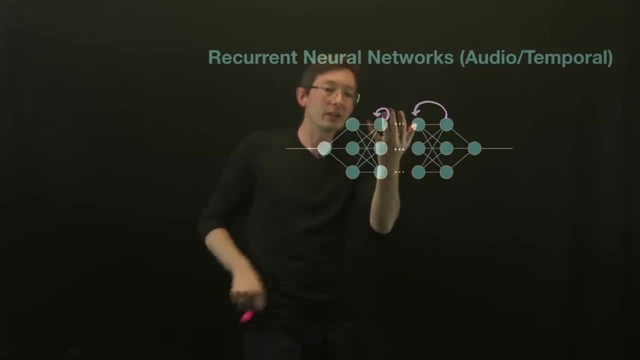 where all of the information just flows from left to right. Here you have this kind of feedback network, this recurrent neural network that gives you this memory. So LSTMs- long, short-term memory networks- are really useful for audio processing and dynamical systems. 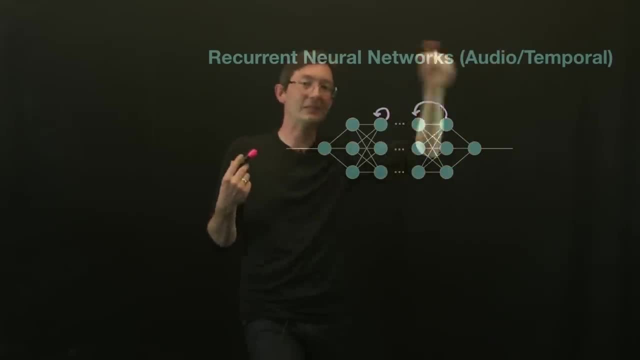 anything that varies in time, Because they have these kind of feedback signals which allow you to have kind of memory. So there's information that's just living here, kind of getting recirculated through this network. So that's pretty cool. Very, very interesting architecture. 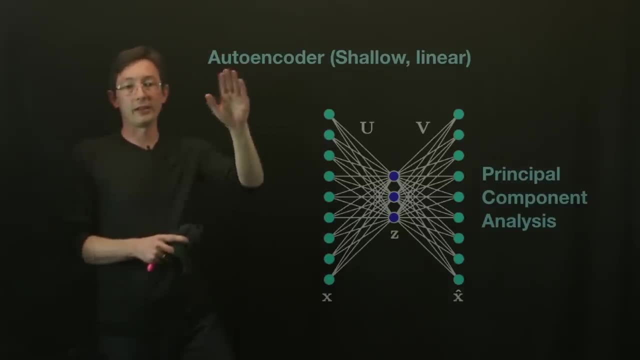 Another one that I really like a lot and I use a lot is the autoencoder. So here I'm showing you kind of what I think of as a shallow linear autoencoder, meaning that my nodes are doing linear combinations, just taking linear combinations of the input layer. 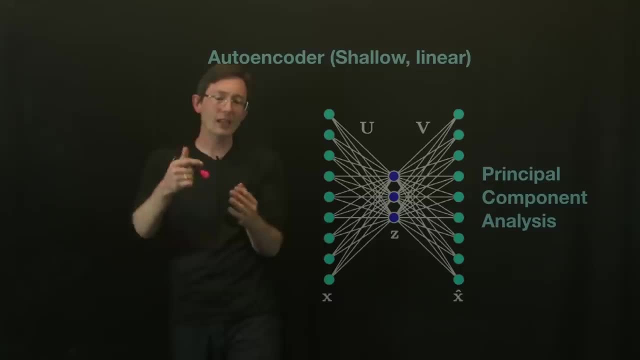 And what the autoencoder is trying to do is take a high-dimensional signal, compress it down to some latent space, this Z variable. that's all the information I need to keep track of in a way that that Z information can be re-lifted back to the high-dimensional image.